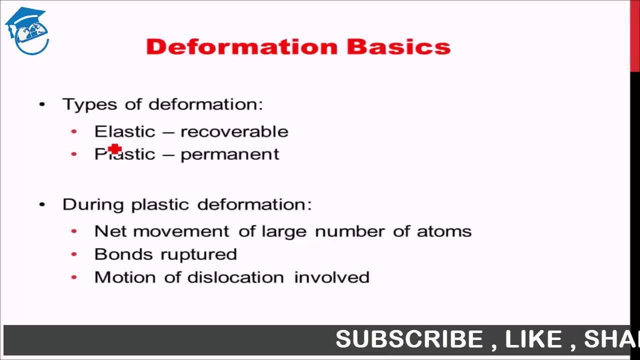 in plastic deformation the bonds actually break, which makes it permanent. Okay. Also, the net movement. as we see here, there is a net movement of large number of atoms which cannot return back to its initial position. Therefore that is permanent in nature. Last, 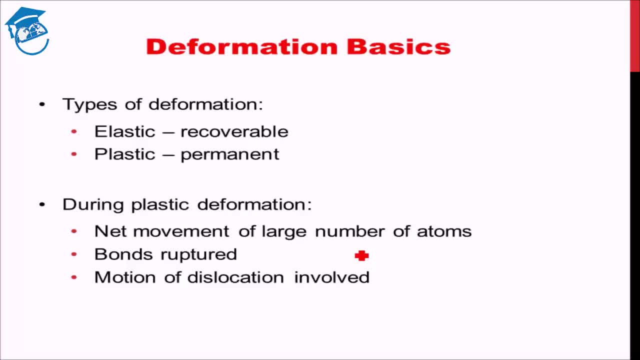 but not the least, the motion of dislocation is the very fundamental concept which drives plastic deformation. We will see that upcoming slides that for the plastic deformation to take place we have to use the plastic deformation. So we have to use the plastic deformation. 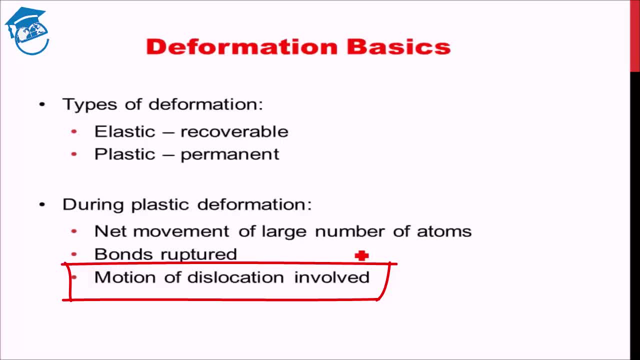 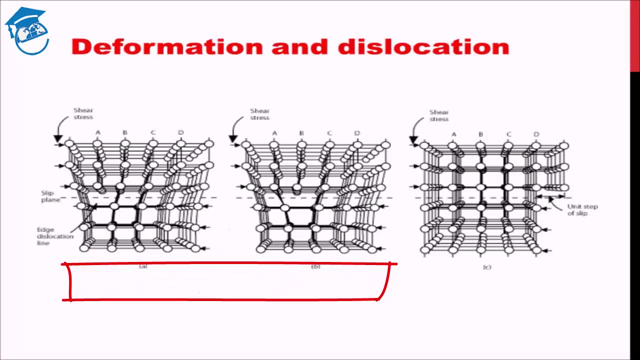 to take place. One of the basic requirement is that there has to be dislocation motion. Dislocation motion is what mainly drives plastic deformation- Dislocation motion. Okay, So now let us see the relation between deformation and dislocation. Here we have shown a edge. 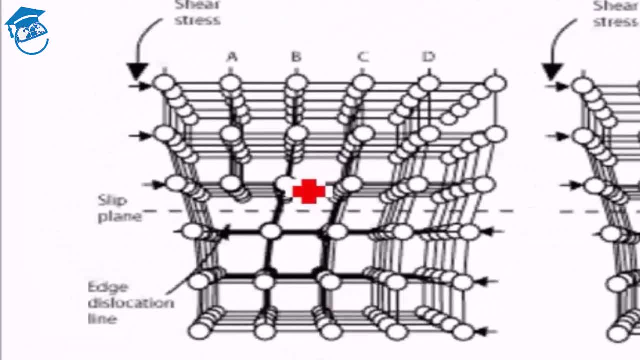 dislocation. We will use the example of edge dislocation. We will use the example of edge dislocation because it is quite easy to visualize what exactly is happening. But the same phenomena, or rather parallel, similar phenomena, occurs in the case of screw dislocation too. And 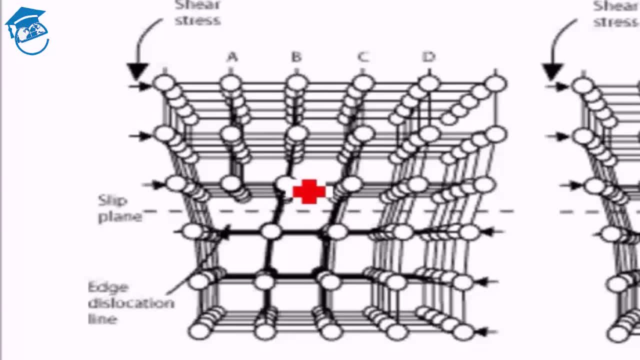 screw. dislocation also leads to deformation. So here what do we have? We have shown five sets of plane here and six sets of atomic planes at the top. So basically, this A set is the extra half plane of atoms, which does not have any extra half plane over here. the 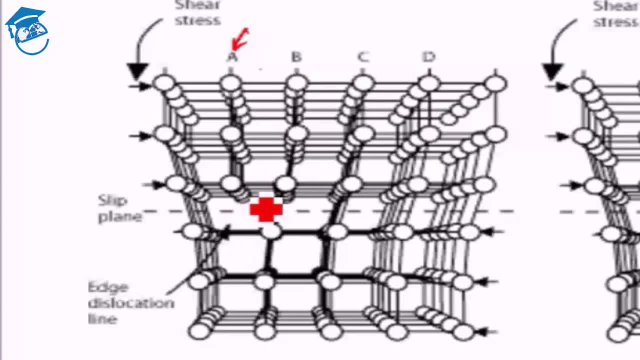 rest of the half plane Now due to- and this is our dislocation line, then This is where the dislocation extra half plane is ending. So this is the dislocation line Now due to this extra half plane. what will happen is that if a shear line is formed, then the 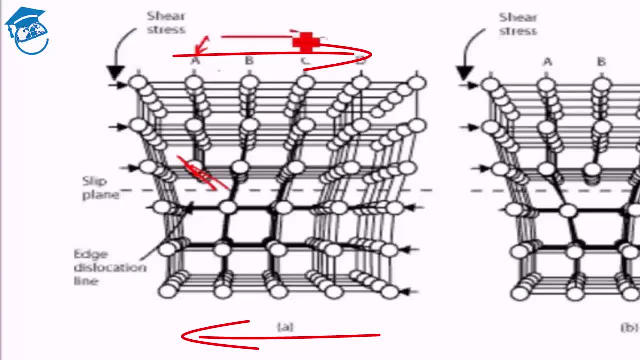 If a shear force is applied, that is, if we apply force like this, a shear like this, These atoms will try move in this direction and these atoms will try to move in this direction. But instead of all the atoms moving in this direction, all the atoms moving in this direction. 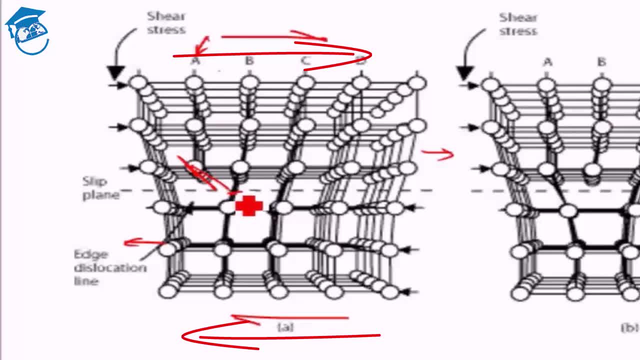 what will happen is that this set of bonds over hereons connecting with the otheris all moving, And which bound will be coming out of the other one is going to connect with this nearby atoms over here? Is this size or size of the natural bond lines? 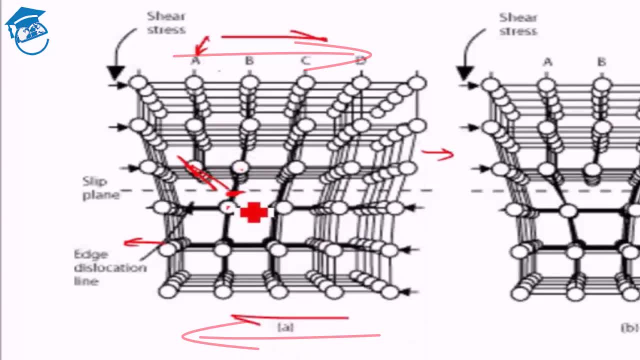 or those vonting� específic bands. This willlà humorize the matter. History of letters using an abbreviated Schüler's law appear. If A force works like this, if the pi", if false force is applied, atom and this atom and the atoms behind those atoms will break And instead of these bonds, 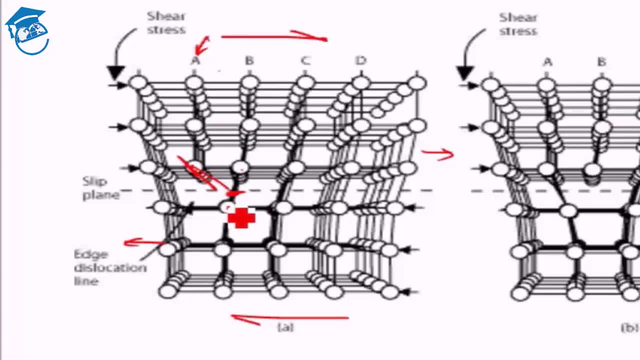 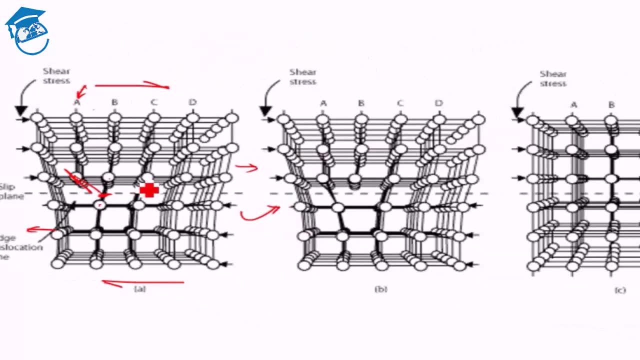 new bonds will be created with these atoms. Okay, so what scenario will give rise? We will get this scenario from this scenario. So, basically, these bonds break, The dislocation seems to move from this location to this location. The extra half plane seems to no longer exist. 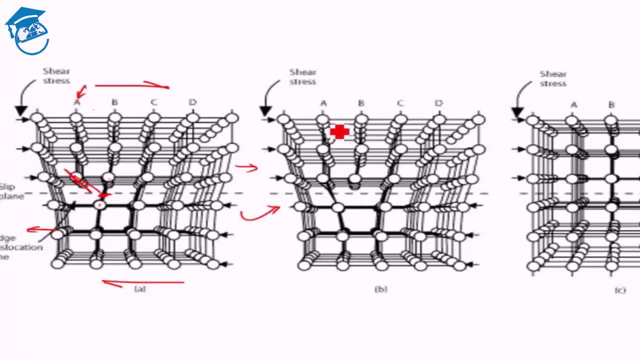 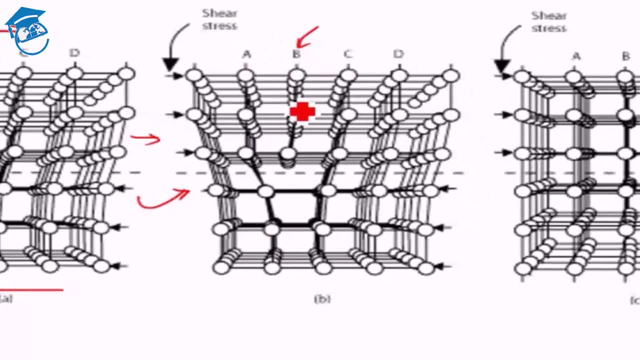 here and move here. Okay, see here, The extra half plane now is no longer the extra half plane. Rather B becomes the extra half plane because these bonds are broken and joined over here. The next step what will happen is this bond will break and join here, so the 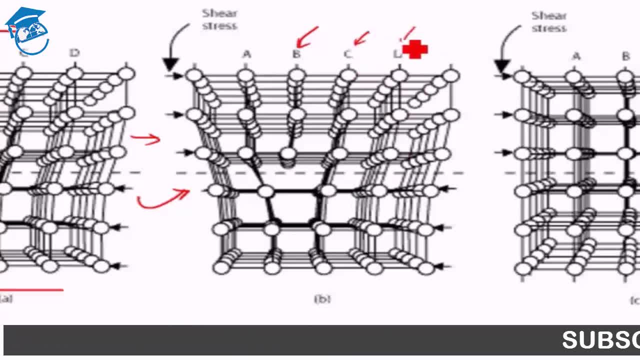 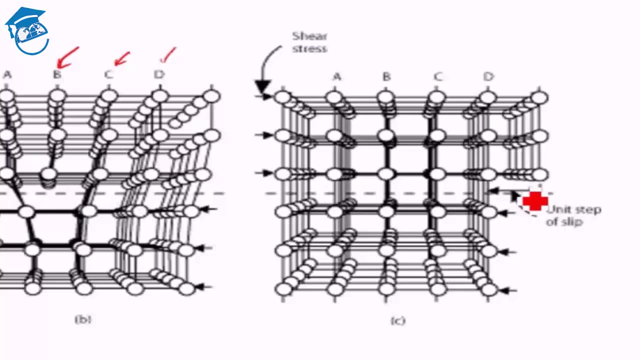 extra half plane comes true To C, then to D. This way, the dislocation line keeps on moving in this plane till it reaches a surface or a grain boundary. Okay, so, ultimately, what will happen is this configuration: It will reach an edge, a surface, and we will get a step here. We will get a unit step here. 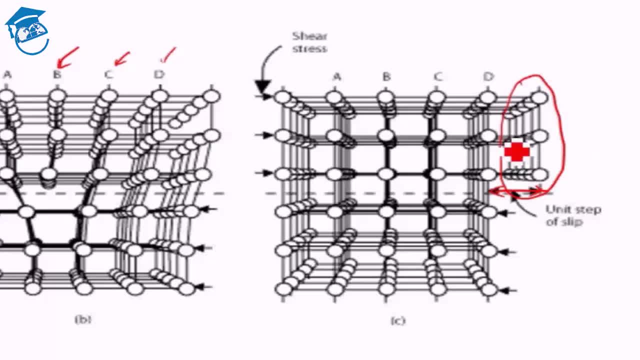 The extra half plane resides here on the surface, which can be seen under a microscope. If you observe it under a microscope, you can see that And these planes are no longer extra half planes. There is no extra half plane within the bulk anymore. 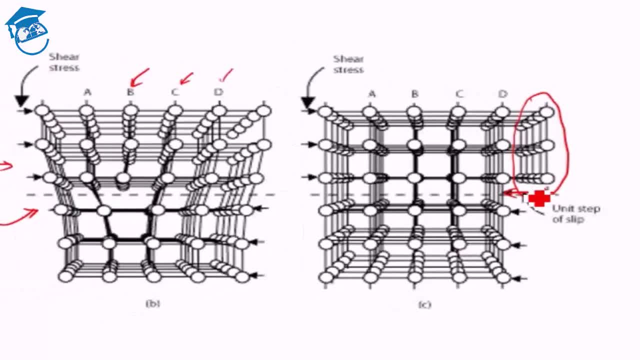 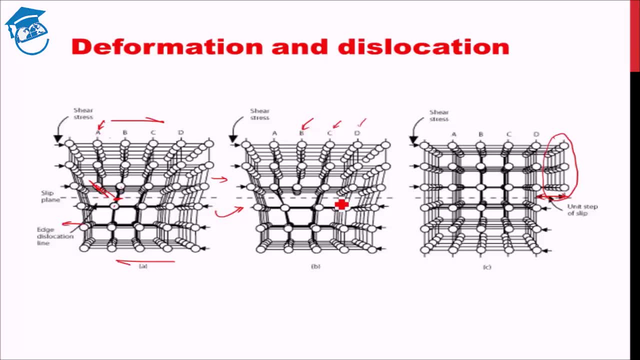 That has reached the surface, that has surfaced, And this way the dislocation motion gives rise to a deformation. right, And this was the case of one single dislocation, But in a real scenario, there are millions and millions of dislocations. 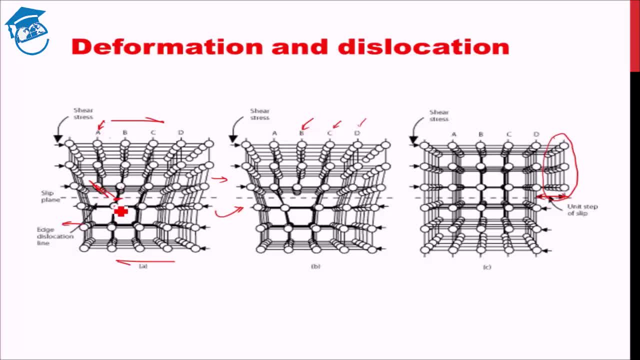 When shear is applied, all those dislocations come into play. And once they come into play there is the bulk effect: Lot of dislocations moving and the effect of each dislocation movement adds up. thereby proper plastic deformation can be observed due to dislocation motion which is taking. 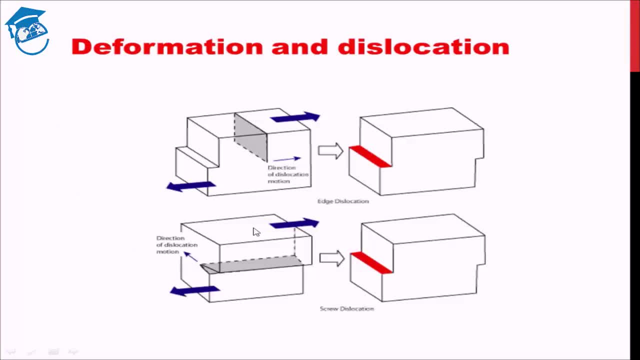 place. Here we have presented the picture in a different way. Here what we have is: top is edge dislocation, Bottom is screwed up. Here we have the edge dislocation In the edge dislocation. if we apply a shear stress like this, what will happen is that: 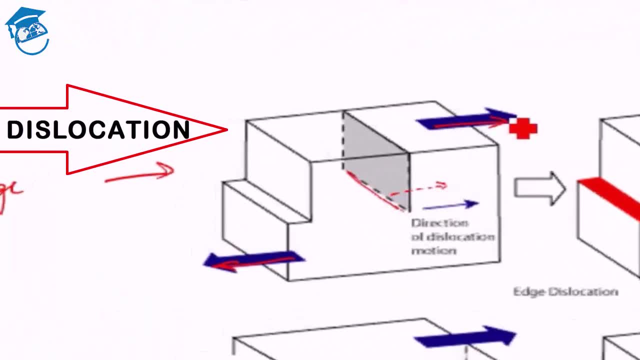 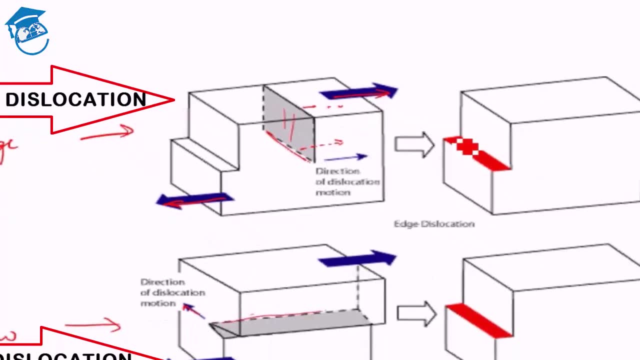 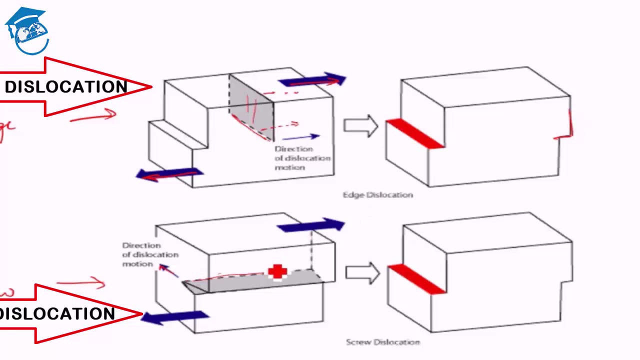 this dislocation keeps on moving due to the shear stress. This extra half plane keeps moving one step at a time, ultimately reaching the surface, and we get a edge here. This is the same thing which we saw in the previous slide To visualize the screw dislocation. the idea is that the screw dislocation is like this: 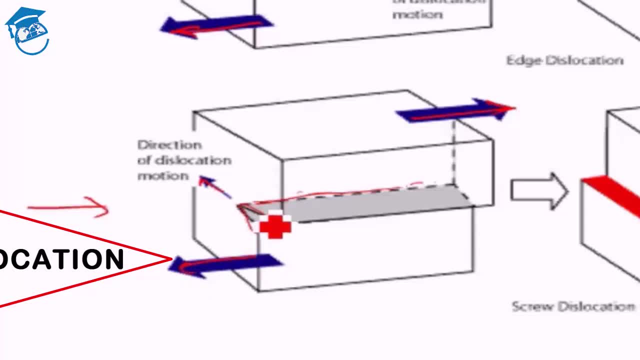 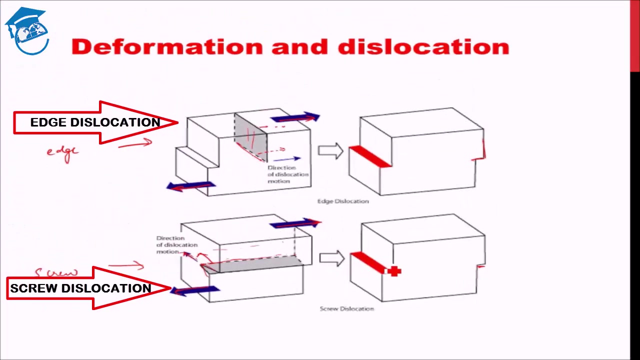 Okay, If we apply a shear, this screw dislocation will move in this direction, perpendicular to the shear, And that will result: this dislocation line will ultimately come till this surface and we will get a step over here and a step over here. So, basically, the dislocation line, the screw dislocation line, has moved in this direction. 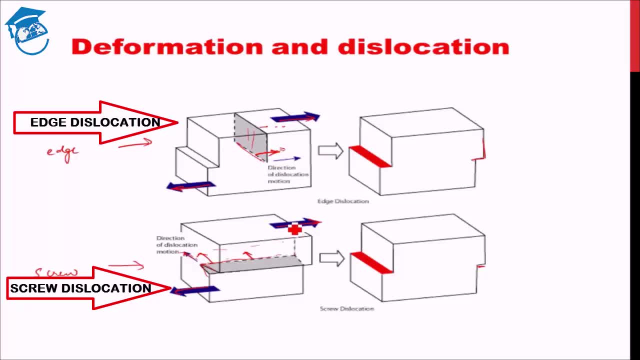 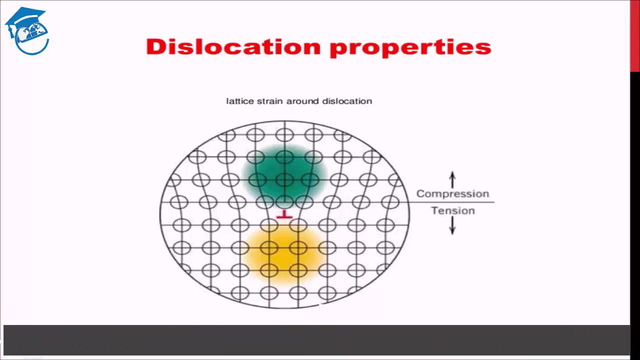 The edge dislocation line has moved in this direction, Though the shear forces were in the same direction in both the cases, And ultimately both of them gives rise to similar structure or similar kind of deformation. Okay Now, in the case of a dislocation, the presence of dislocation leads to a stress field. 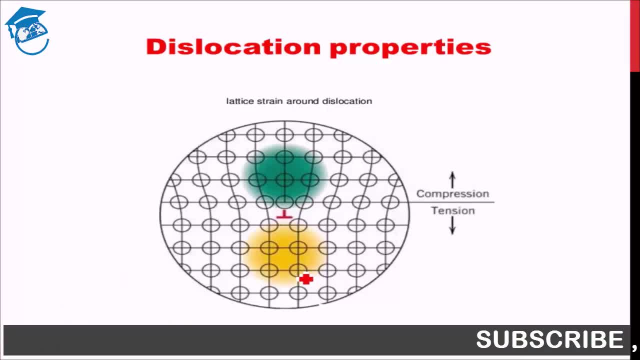 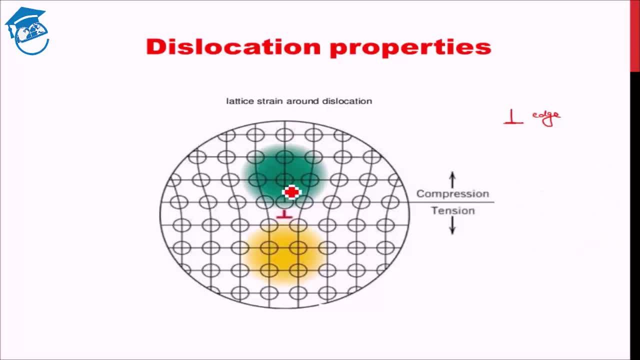 positive edge dislocation, That is, the extra half plane is on the top. There is no plane corresponding at the bottom, which means at the top we have more number of atoms squished in same amount of area here, Less number of atoms squares in that area. 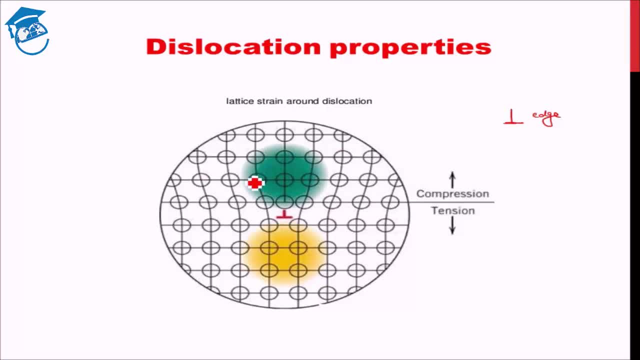 Since there is more number of atoms here squeezed in a given area, there will be atoms pushing against each other, That is, there is compression forces developing here. So where the extra half plane is present, there will be compressive lattice strain development. So here there is compression forces. 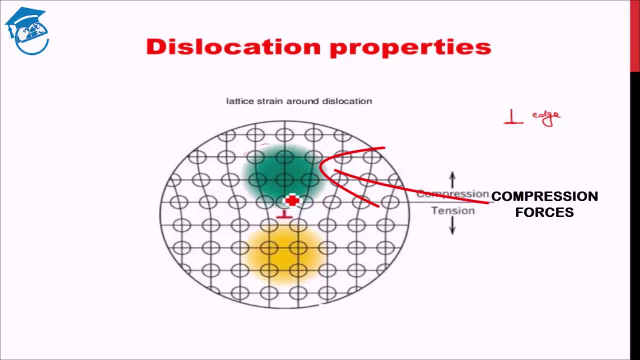 Closest to the extra half plane, the amount of compression is the maximum. As we keep moving outward from the extra half plane, the magnitude of compressive force keeps on reducing And at a very far distance it fades to almost zero, Whereas at the bottom half, where the extra half plane is missing, there are less number. 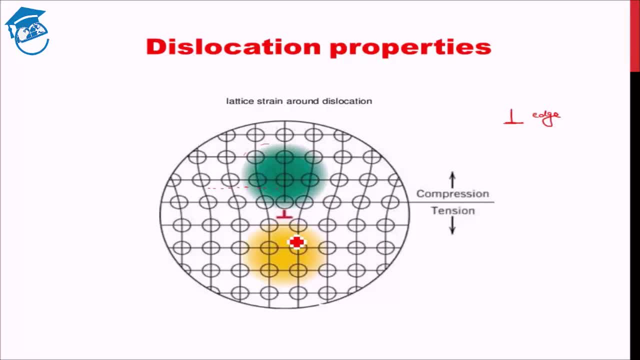 of atoms, Thereby more space is available. As a result, there will be tension forces here. The atoms will try to pull each other, Because more space is there, less number of atoms are there. So the absence of extra half plane results into tension forces. 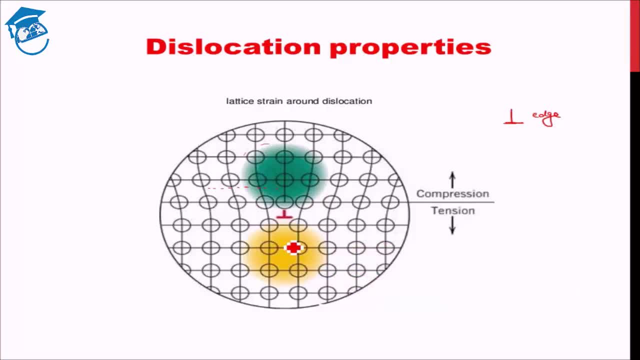 Okay, This idea, the idea about the lattice strain around a dislocation, is quite fundamental because this will help you understand The interaction between dislocation and dislocation, The interaction between dislocation and solute particles. This will help you understand the different strengthening mechanisms which we will see. 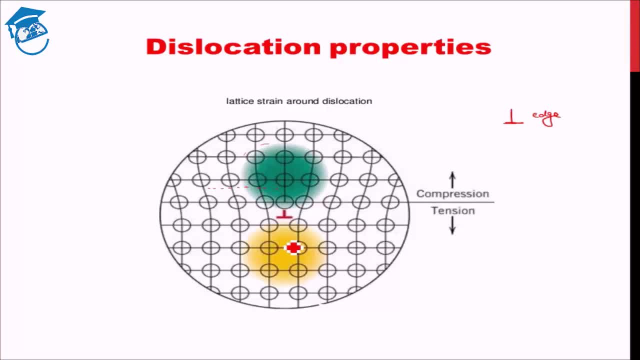 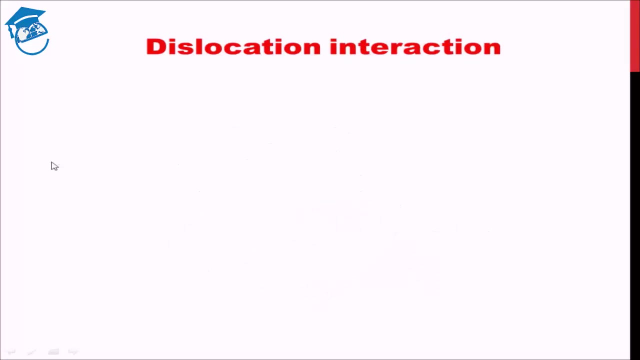 in the future lectures. So be quite clear with this that the presence of extra half plane leads to compressive forces. The absence of extra half plane leads to tensile condition, tensile strain. Okay, Now Let's see what are the dislocation interaction taking place.